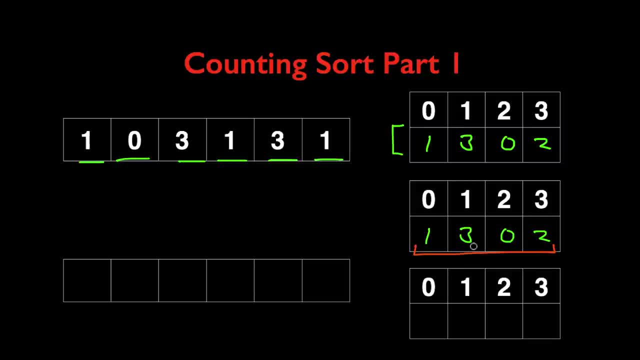 occurrences for each number. the second step is going to be adding each number to the right of it accumulatively. What I mean by that is the first number at index, 0, stays the same, and the second number will be: 1 plus 3 equals 4, and the third number will be 4 plus 0,. 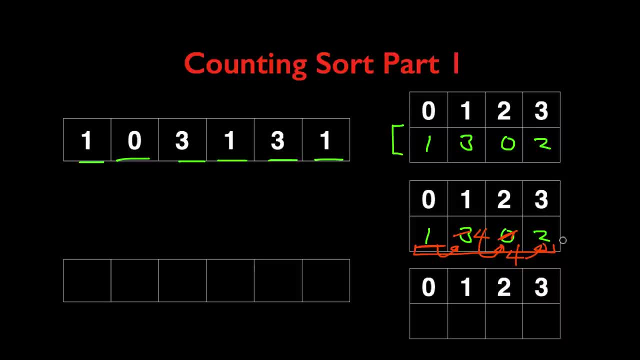 which is equal to 4, and the fourth number at the index, 3, will be 4 plus 2,, which is equal to 6.. After that step, we have the numbers 1,, 4,, 4,, 6. for the numbers 0,, 1,, 2, and 3.. 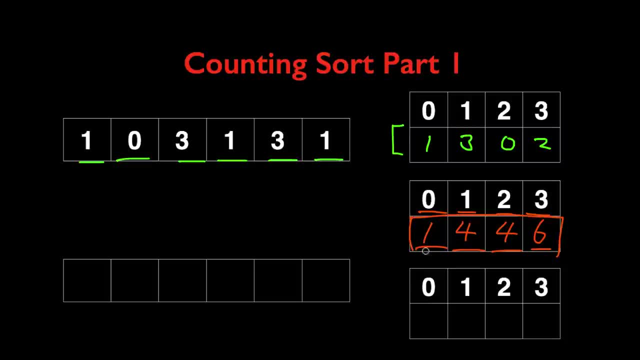 The next step is going to be shifting this whole array to the right by one cell, and we're gonna do that by looking at this array from right to left. We're gonna first start with the last index, which is index 3 in this particular case, and the value. there should be the value. 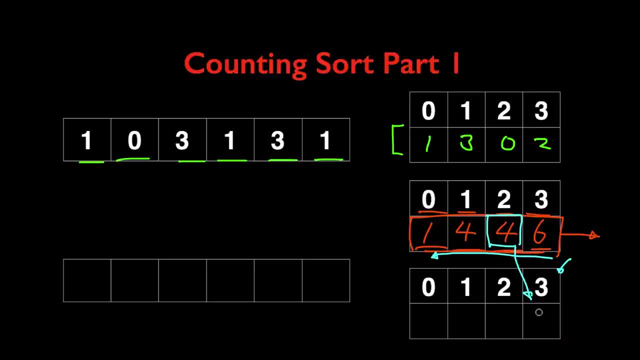 that's currently in index 2, so we're gonna put 4 at index 3.. And we're gonna do the same thing for index 2.. The value here should be what's in index 1 currently, so it should also be 4, and at index 1, we're gonna put 1.. At index 0, we're gonna put 0.. And these 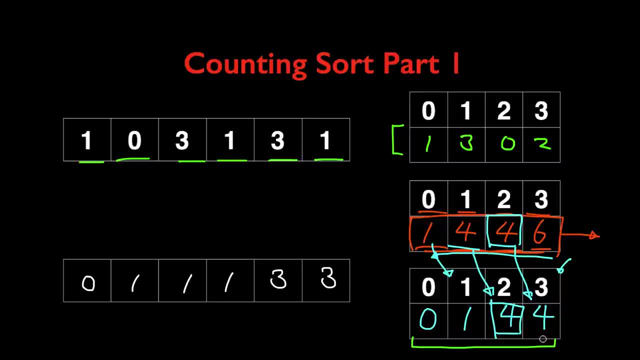 These numbers- 0,, 1,, 4,, 4, are actually the starting indexes for the range of numbers we have in this particular case: 0,, 1,, 2, and 3.. And here's one way to think about it. 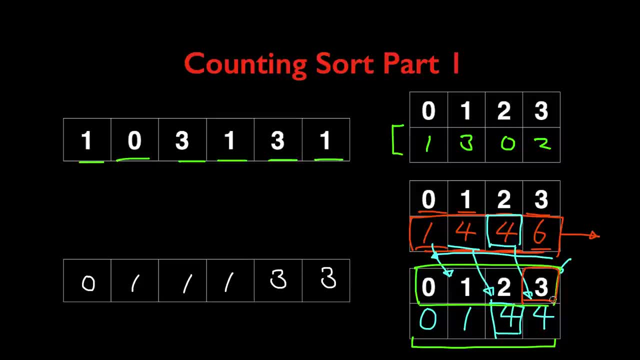 If you look at the number 3, or the index 3,, the corresponding number, the corresponding starting index is 4.. And that's because, when we sort this array, the number 3 will start at the index 4.. Another way to think about it is that there are four items that should appear before the 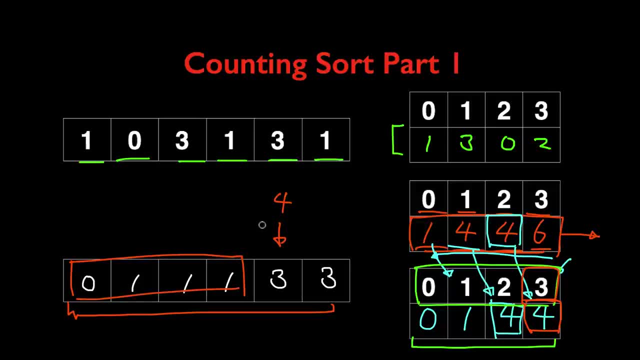 number 3 in the sorted array, And that should be obvious. if you just look at the first array that we constructed, There's one occurrence of 0,, three occurrences of 1, and zero occurrences of 2, so, adding them up, there are four items that should appear before the number 3, and that's why. 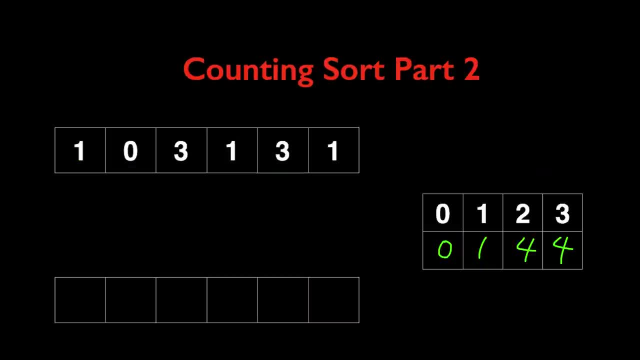 the starting index for the number 3 is 4.. Once we have the starting index for each number, the rest is relatively easy. We're going to first initialize a new array that's the same length as the original array, so length 6 in this particular case. 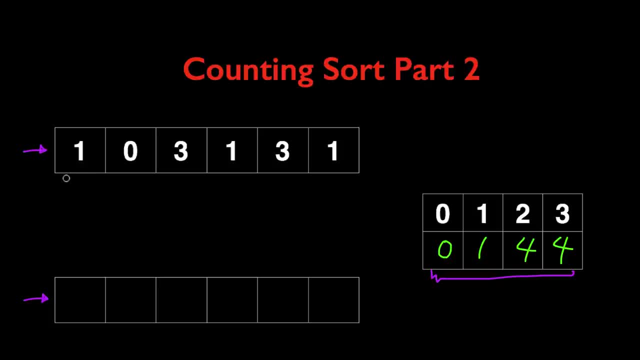 And then we're going to iterate through the original array one by one. When we are looking at the first element of this array, which is 1,, we're going to check what the starting index should be for this number from the array that we constructed. 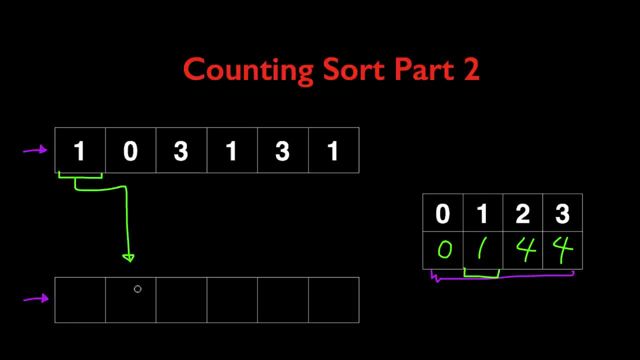 We see that the starting index should be 1.. So we're going to put this number into index 1 of the new array, And then we're going to increment our starting index by 1, and it becomes 2, and this is. 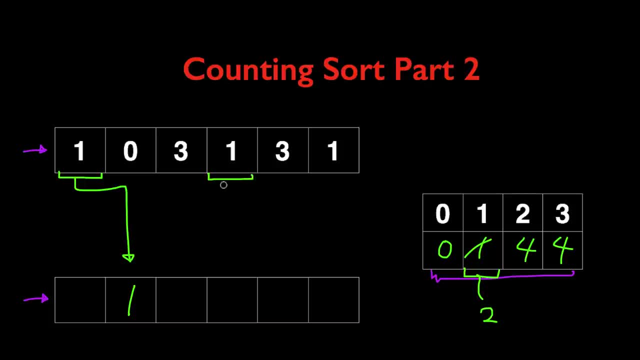 so that when we look at the second instance of the number 1, we'll know that it should go into the index 2 instead of 1.. And then we're going to increment it again. We'll do the same thing for each number of this array, from left to right, until we get. 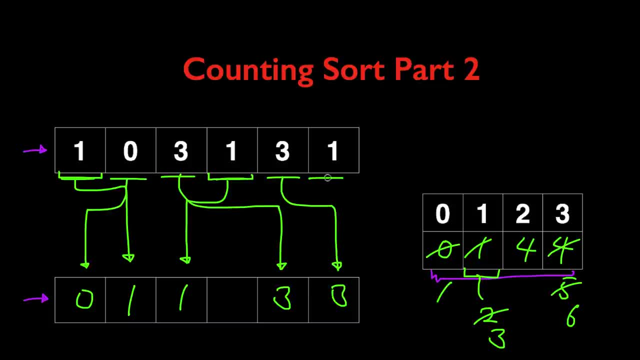 to the last number in the original array. Now you might have noticed that this process makes counting sort a stable sorting algorithm. What that means is that, of course, if you look at different instances of the same value, for example the number 1, the order in which they appear in the new sorted array is exactly. 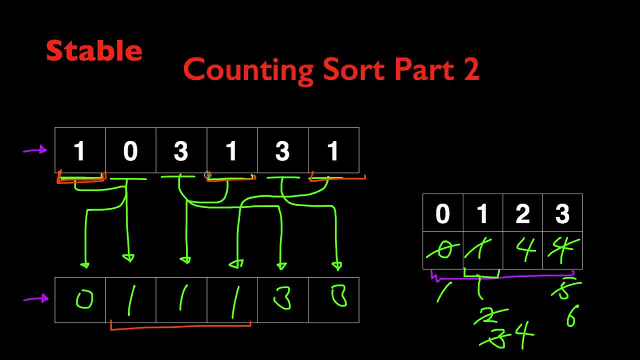 the same as the order in which they appear in the original array. This wouldn't matter if they were just number 1, but if they represented underlying meanings to them, For example, if they were ages of people, three different people, let's say Emily Tom. 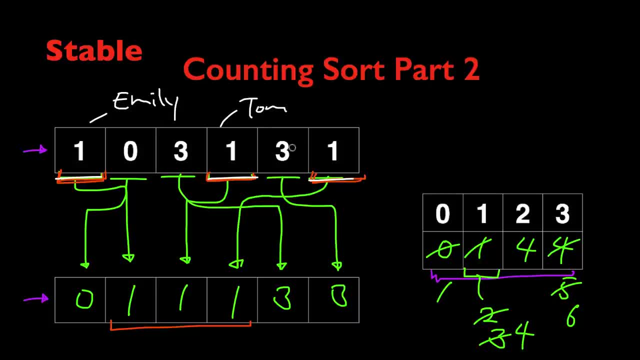 and George, then we might care if they appear in the same order or in a different order in the sorted array as the original unsorted array. Now let's quickly go through a few important properties of counting sort. First of all, as I mentioned, it's a standard. 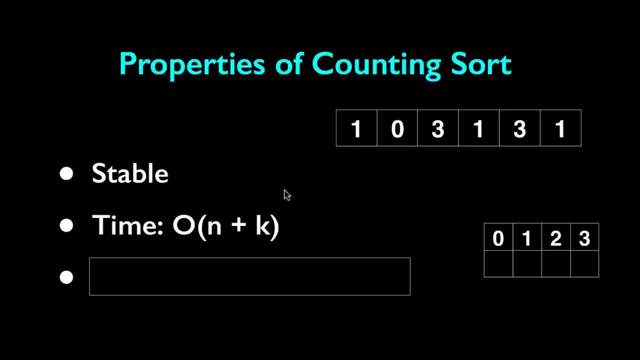 It's a standard, It's a stable sorting algorithm And the time complexity for this algorithm is bigger than n plus k, where n is the number of items that we have in the original array and k is the range of numbers that we could.